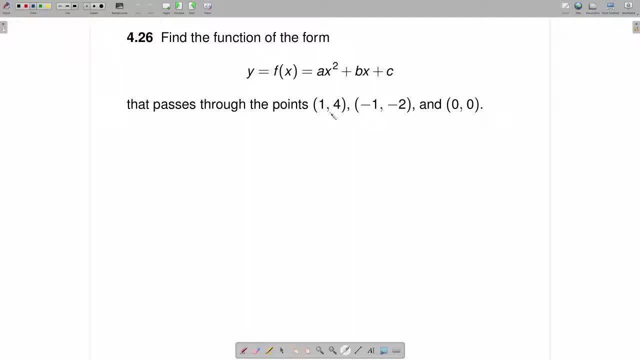 is a quadratic function and we're trying to find the quadratic function. In other words, we're trying to find the coefficients a, b and c that correspond to a quadratic that passes through those three points. You may have heard the saying: two distinct points determine a line. 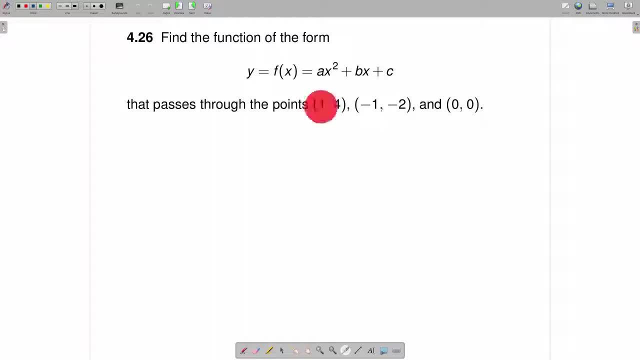 Well, this is the next level up from that, and this is three distinct non-collinear points determine a quadratic. So let's start out with the these three points here and see what the meaning is, What this is saying. when you see 1, 4, is that saying that f of 1 is equal to 4.. 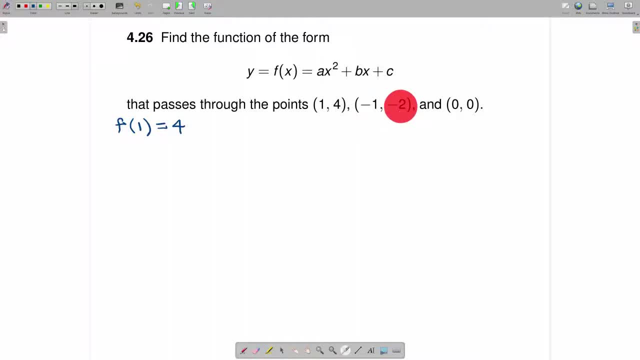 When you see that negative 1, negative 2, that's the same as saying f of negative 1 is equal to negative 2.. And when you see that 0, 0 lies on the quadratic, that's the same as saying f of 0 equals 0.. 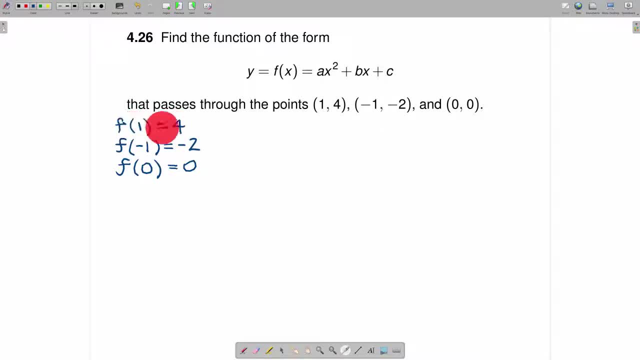 So, taking this first piece here, f of 1 is equal to 4, I'm going to go ahead and write out f of 1 here, And f of 1 turns out to be nothing more than a times 1 squared plus b, times 1 plus c. 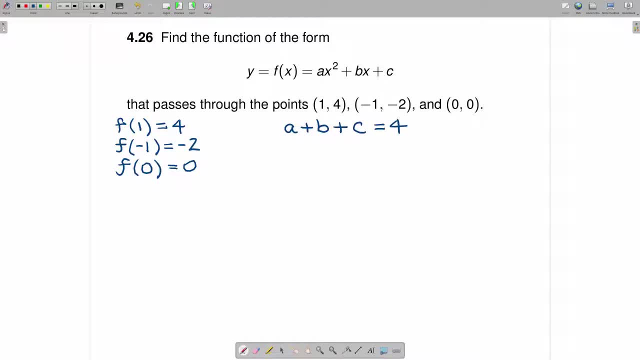 and we know that is equal to 4.. Let's take this second equation: f of negative 1 equals negative 2.. Well, f of negative 1 will be a times negative 1 squared, and a times negative 1 squared is just a. 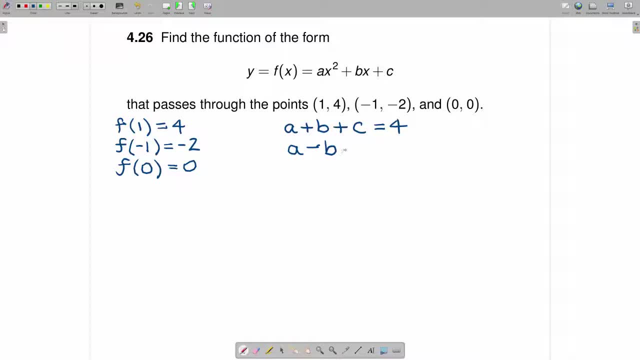 plus b times negative 1, that's going to be minus b plus c is equal to negative 2.. Finally, how about f of 0 equals 0?? Well, in that case, what we have is we have a. 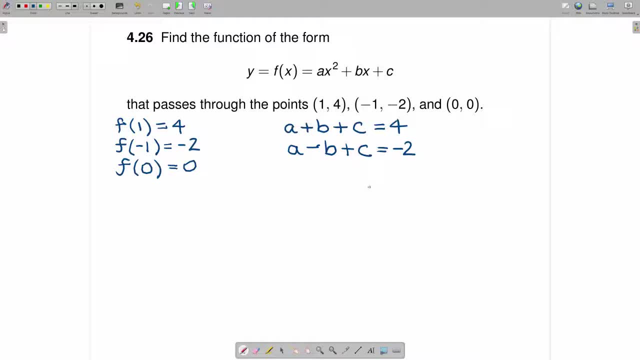 a times 0, squared plus b times 0, plus c, is equal to 0. So what we have here is we have three equations in three unknowns and we need to solve those equations Now. we're very fortunate because this third equation is already solved for c. 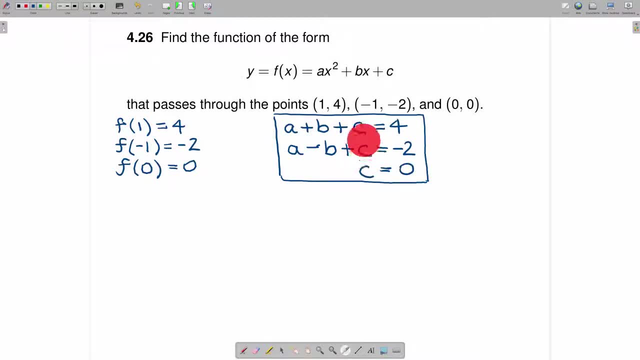 So we can take this c equals 0 and plug it into these first two equations, and then we will have reduced the system of equations to a plus b plus 0 equals 4, and a minus b plus 0 is equal to negative 2.. 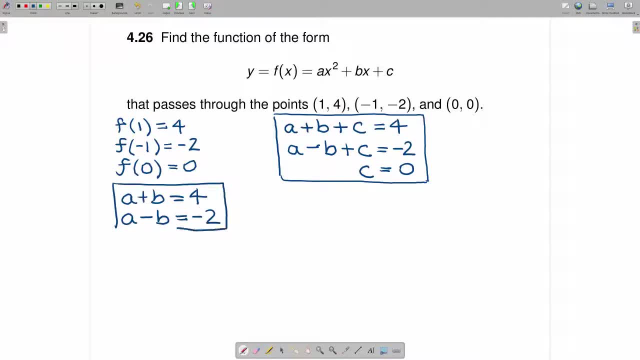 So we already have one of the variables solved for in the first set, c equals 0, and so what we did was we plug that c equals 0 into these two to reduce it to a system of equations, that is, two equations and two unknowns. 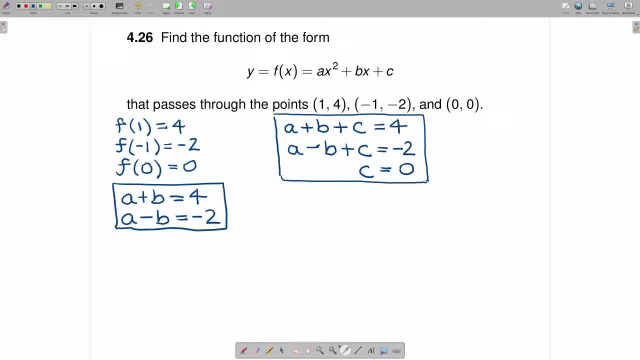 Well, the next step here is to solve this two by two system of equations, and one thing you can do- this is called substitution- is we can solve this bottom equation for a and then everywhere there's an, a in the top equation. 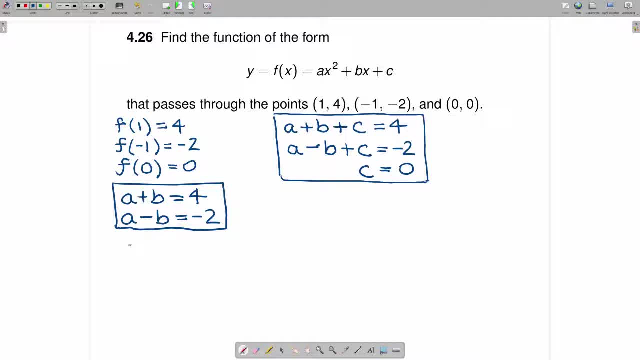 we can plug that in. There's a lot of different ways to solve it, but this is one way. So we can take a minus b is equal to negative 2, and we can solve that for a. The way you solve that equation for a is you add b to both sides of the equation. 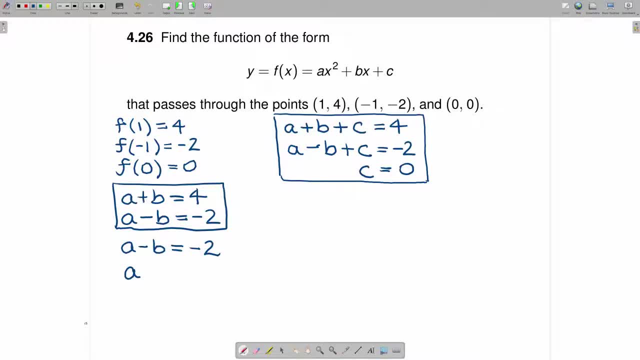 So when you add b to the left hand side of the equation, you just get a. When you add b to the right hand side of the equation, you get b minus 2.. So now we know that a is equal to b minus 2,. 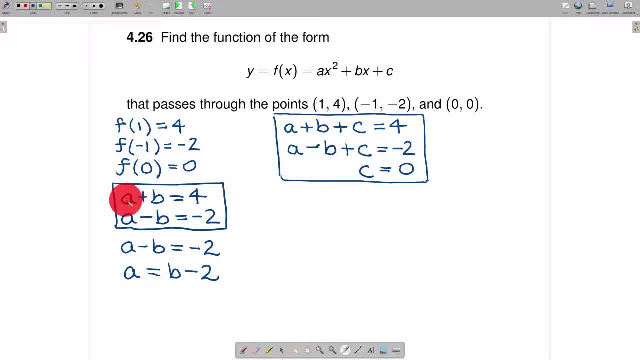 and we can now go up to the top equation and everywhere we see an, a plug in b minus 2.. So let's do that here. So now what we have is we have b minus 2, that's the a plus b is equal to 4.. 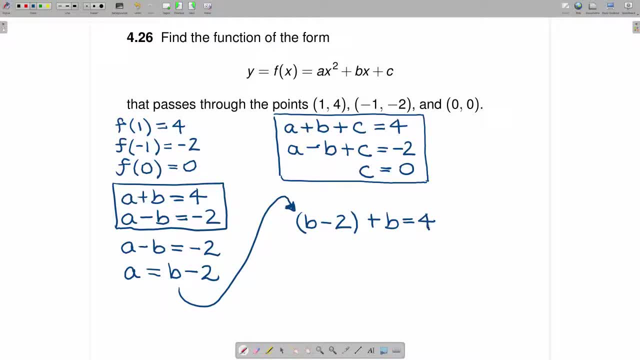 So we would like to solve that equation and we see that we have b plus b, so that is 2 times b minus 2 is equal to 4.. Next step is to add 2 to both sides of that equation. When you add 2 to the left hand side of the equation, 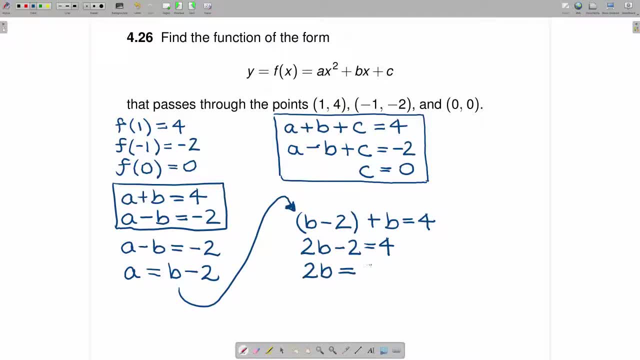 you get 2b. When you add 2 to the right hand side of the equation, you get 6.. Finally, the last step to solve this equation is divide both sides by 2.. When you divide the left hand side by 2,. 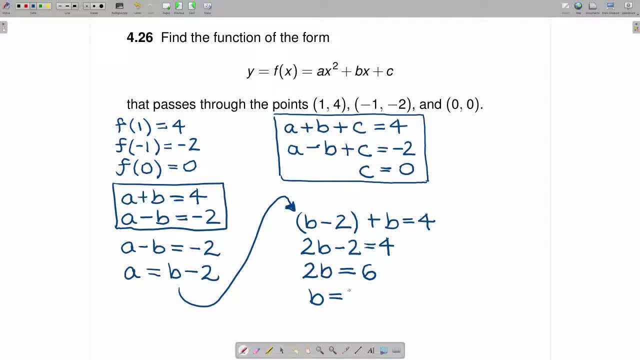 you get b. When you divide the right hand side by 2, you get 3.. Now, at this point, we have c and we have b. The only thing that is missing is a. So we can take this: b equals 3,. 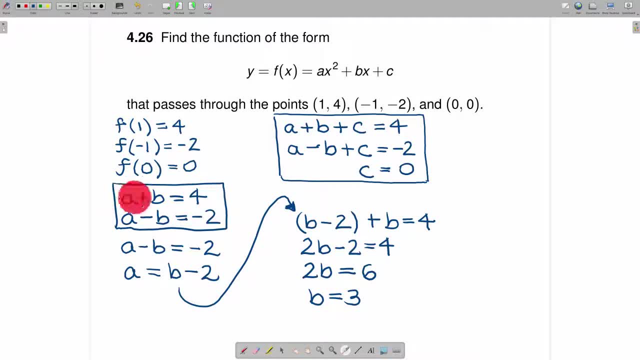 and we can plug into either of these two equations. Let's just choose the top one: a plus b is equal to 4.. That avoids any negatives. So the next step here is to say a plus b, and b happens to be 3,. 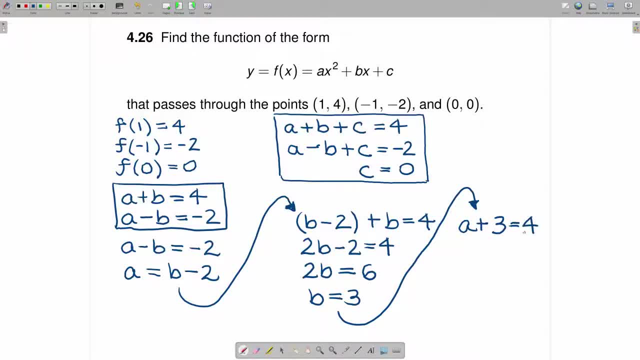 is equal to 4.. The way you solve that equation for a is: you subtract 3 from both sides. When you subtract 3 from the left hand side, you get a. When you subtract 3 from the right hand side, you get 1.. 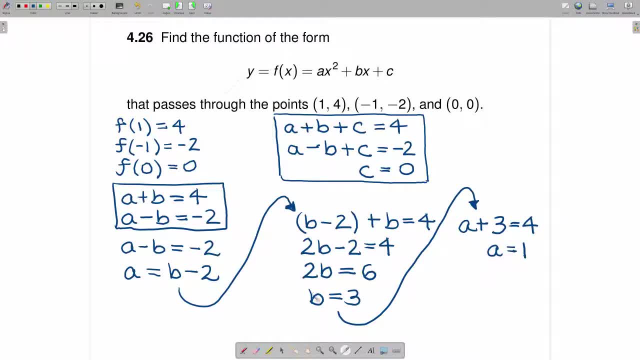 So now we have all three pieces: a is equal to 1,, b is equal to 3, and c is equal to 0. So to answer the question, I want to find the function of this form that passes through those three points. 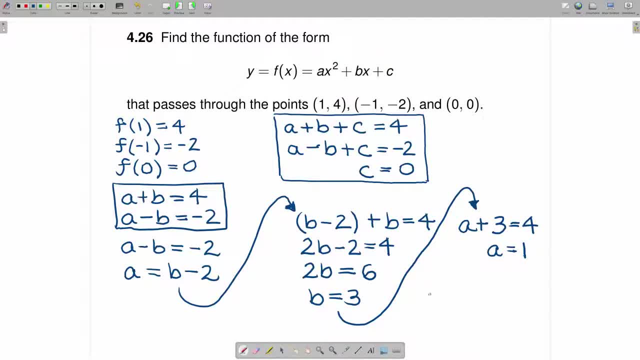 I have my a, b and c so I can write down that answer. So the solution in this case will be: y is equal to f of x is equal to a, which is 1, times x squared. 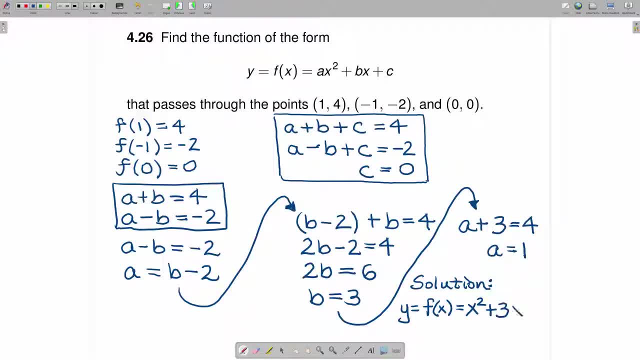 plus b, which is 3, times x plus c, which is 0. And that is the quadratic function that passes through these three points. And if you wanted to go back and check, you could plug in and make sure that with this function right here.